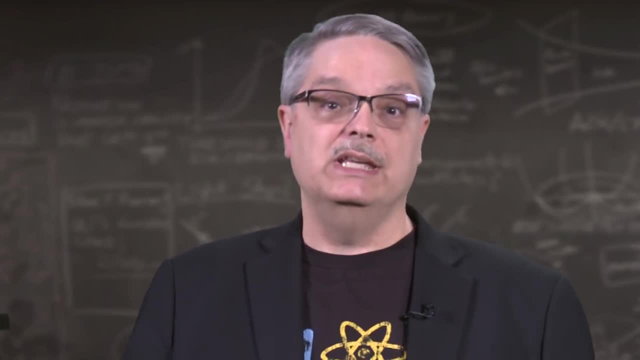 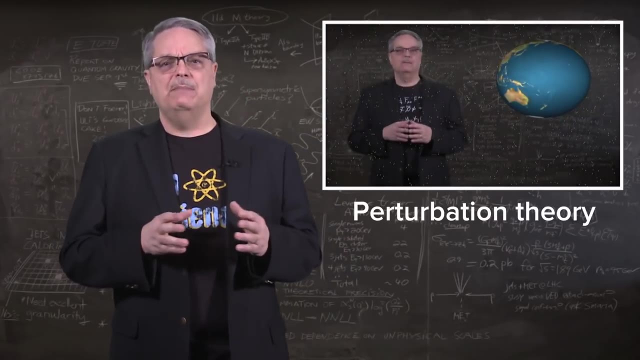 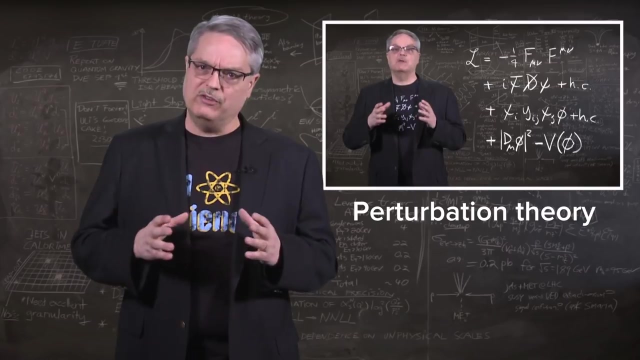 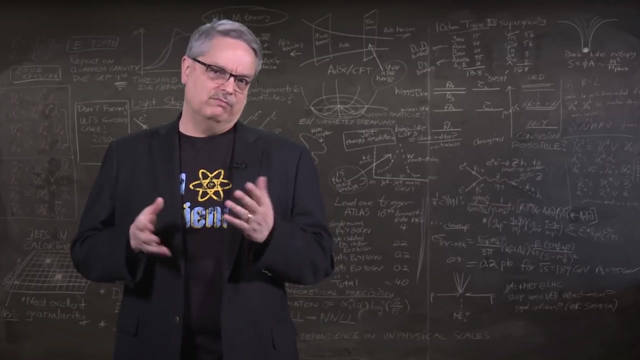 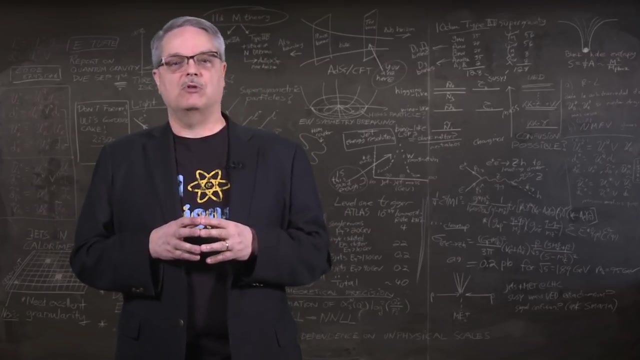 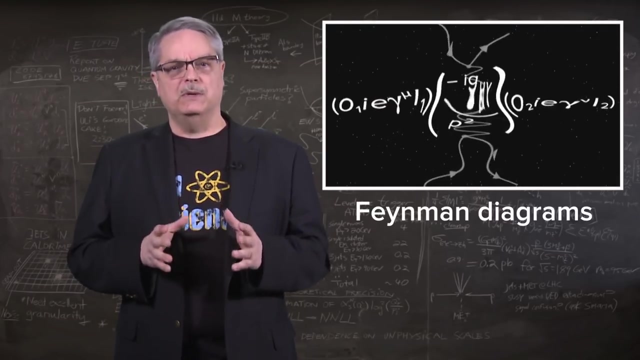 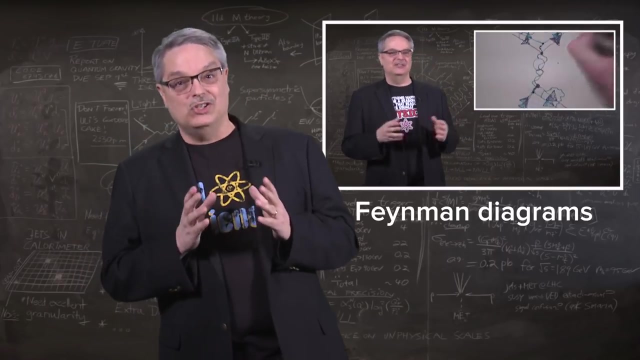 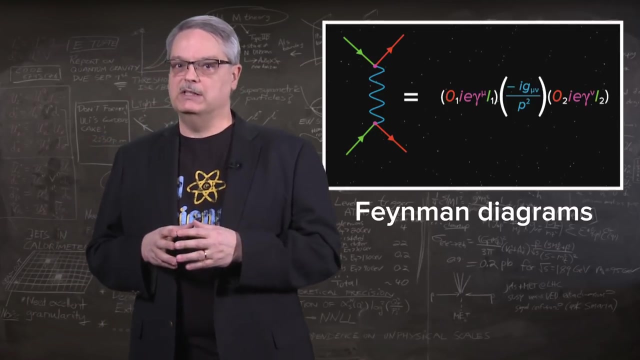 Now before we get into that in a big way, I should let you know that to do a QED calculation depends on two crucial components. The first is an idea called perturbation theory. I made a video that talked about that in detail, and it would help you if you watched it. But the basic idea is that if you are confronted with an equation that is too difficult to solve, you replace it with an approximate equation that is easier to solve. As long as the correct and approximate equations are similar, you will get a reasonably correct answer. And if you need a more accurate calculation, you just use a more accurate approximation. The second idea is that every Feynman diagram that you see is really just a pictorial depiction of an equation. I made yet another video that goes into that in a deeper way. But for right now, just remember that when you see a diagram like this, it is actually standing in for an equation, and every diagram has a corresponding equation. 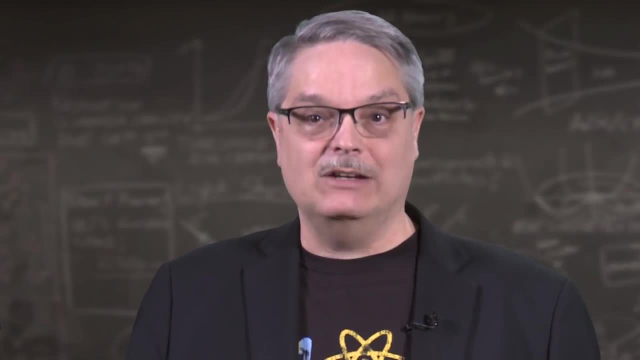 Okay, so with those ideas out of the way, what we can now do is talk about QED. 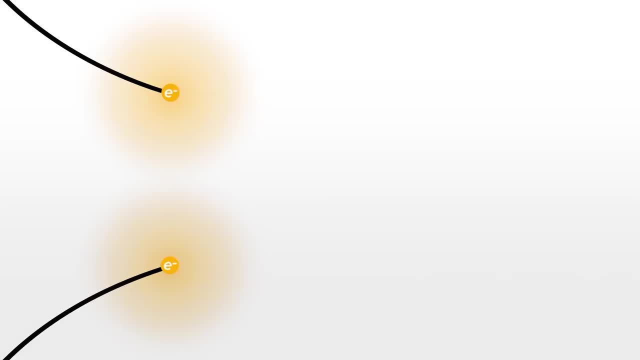 So suppose you wanted to simply calculate how two electrons scatter when you shoot them at one another. If you have any classical physics training, you'll no doubt think in terms of an electric field pushing the two apart. How do you do that? Well, if you have any classical physics training, you'll no doubt think in terms of an electric field pushing the two apart. How do you do that? Well, if you have any classical physics training, you'll no doubt think in terms of an electric field pushing the two apart. However, this is, after all, quantum electrodynamics, so we're governed by quantum effects. And one of the big things here is that the electric field is now quantized. Rather than a big and amorphous force field, the electric field is created by a series of individual and discrete photons. 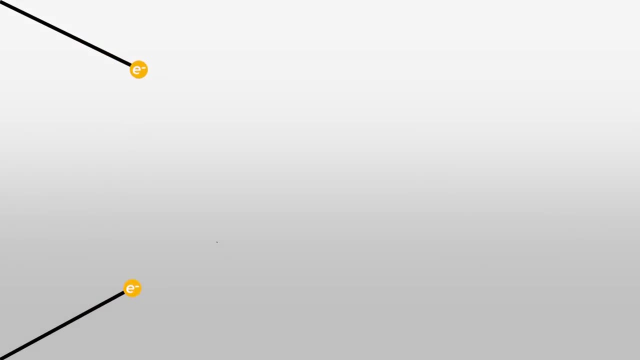 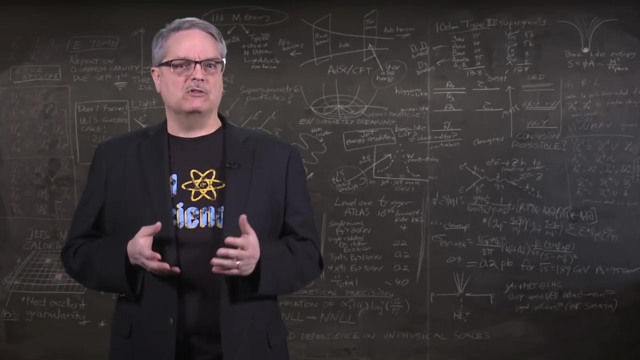 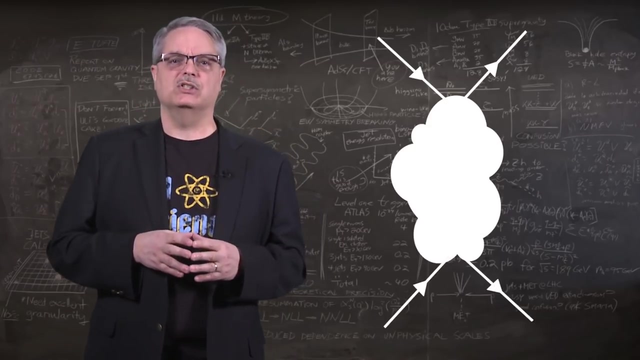 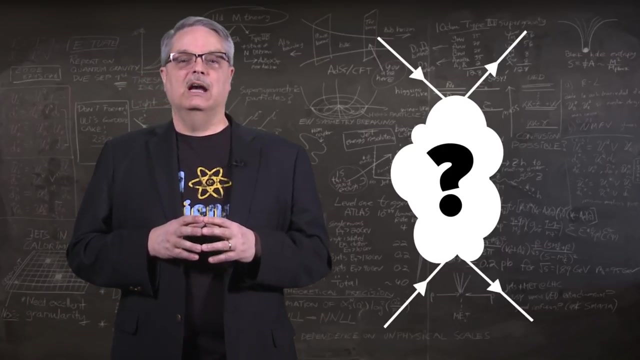 Thus the right way to think about the scattering between a pair of electrons is that the two particles exchange one or more photons. As one electron emits a photon, it recoils, as does the electron. If multiple photons are emitted and absorbed, the outgoing electron trajectories will reflect the contribution of all emissions. Since we don't know in any specific scattering between two electrons what's going on, we can sort of draw it like this, with electrons coming towards one another and then leaving the interaction, with an amorphous blob that indicates our ignorance of exactly what is going on in the collision. 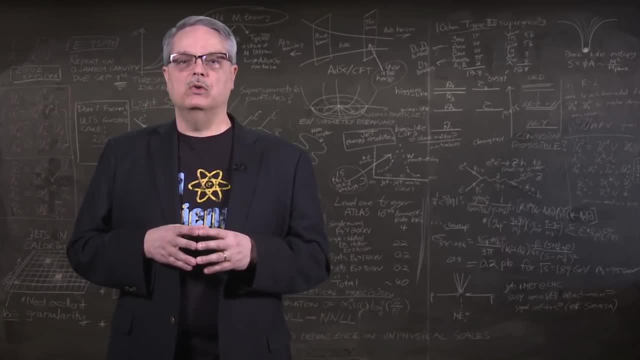 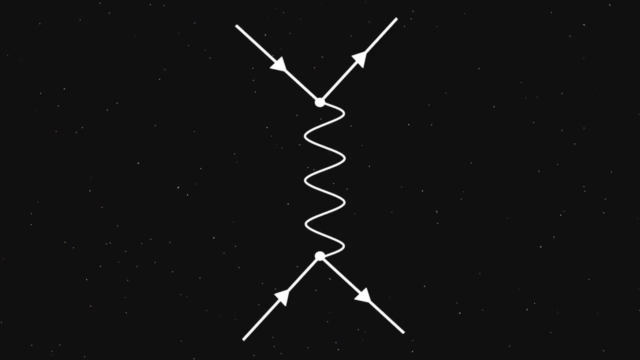 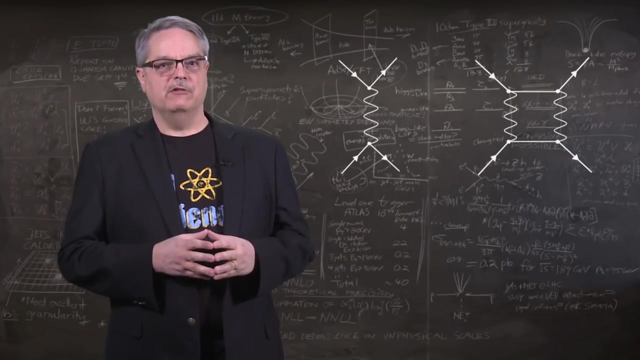 However, what we can do is employ Feynman's equations. We use Feynman diagrams to show that what the blob represents is actually just the sum of all things that are possible. To orient you, the wiggly lines here are photons, while the straight ones are electrons. We have the situation of one photon exchanged. Then there is a situation where two are exchanged. Since we can't uniquely identify which outgoing electron corresponded to which incoming, there are some other diagrams that really should come into play, but we're ignoring them here. After the simplest two diagrams, things get a little bit more complicated. We're going to look at some of these diagrams in a moment. 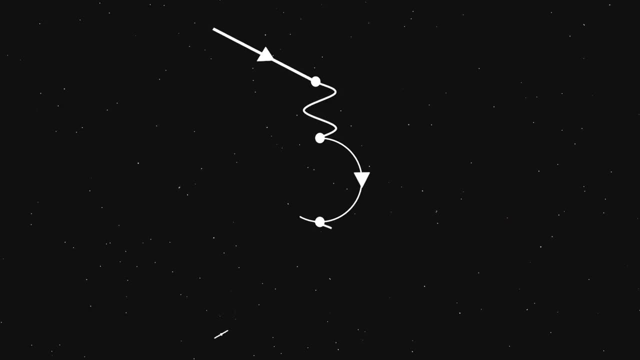 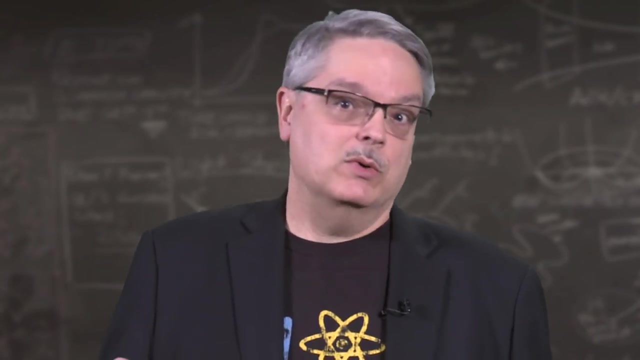 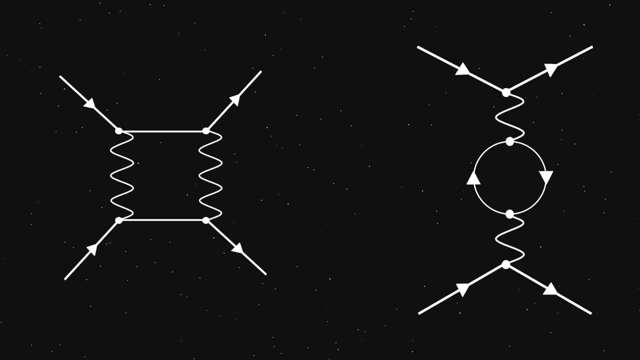 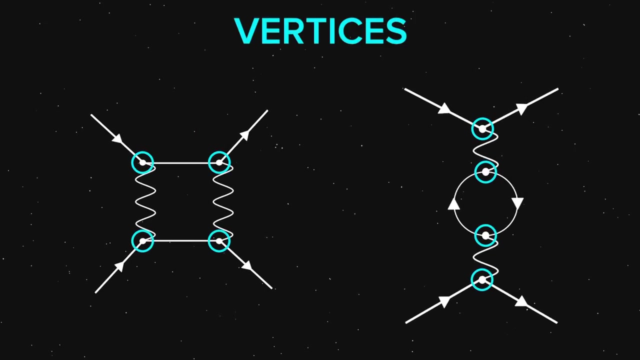 For instance, the photon could temporarily turn into an electron in antimatter electron pair, or while the electrons are exchanging a photon, one of the electrons could exchange a photon with itself. There are tons of other possibilities. So is there a way to simplify this? It probably won't shock you that there is. Remember that I said that these pictures were stand-ins for equations, so I'd like to draw your attention to the spots where the photons are emitted or absorbed. We scientists call them vertices, and they are key to figuring out which Feynman diagrams matter more than others. 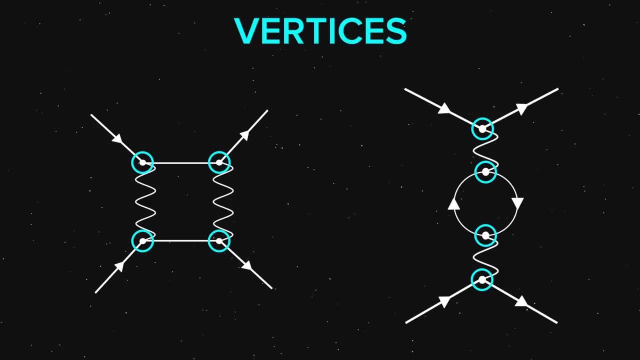 It turns out that photon emission or absorption is hard. Specifically, each emission or absorption 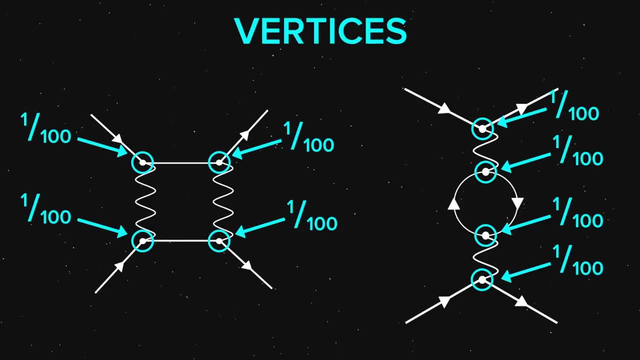 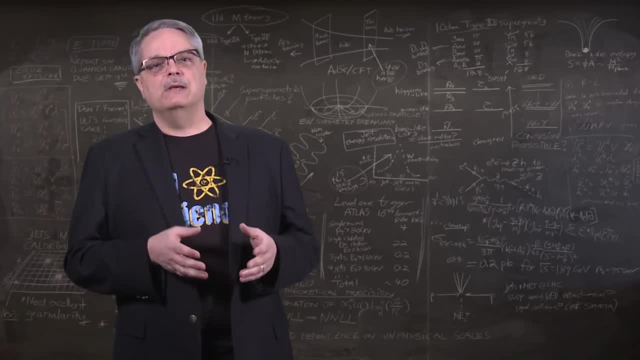 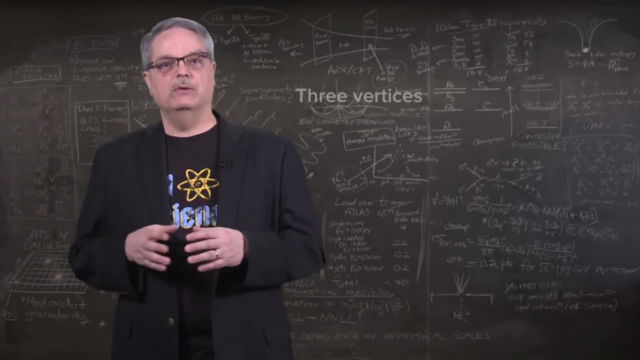 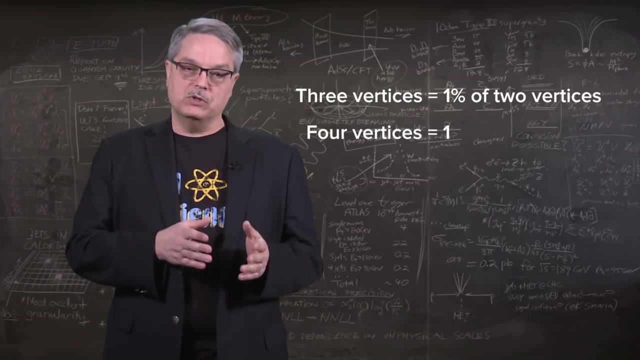 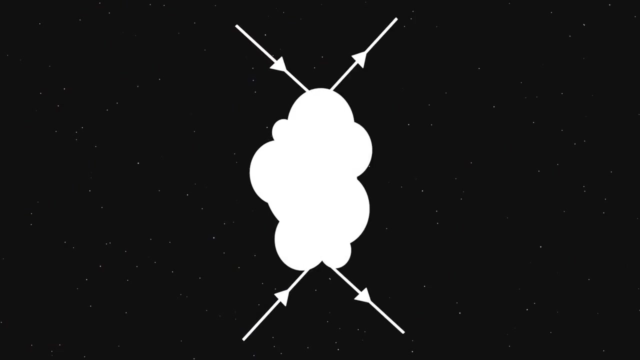 reduces the probability by about a hundred-fold. In practical terms, that means we can simply count vertices and get a sense of how much each diagram contributes. The simplest electron scattering Feynman diagram has two vertices. There are no pictures with three vertices that have two electrons in and two out. They're not very important, because this is just a But if there were, they would happen about 1% as often as the two-vertex case. Four vertices would be 1% of 1%, or 0.01%, etc. Thus we can see that the first and simplest picture really dominates. 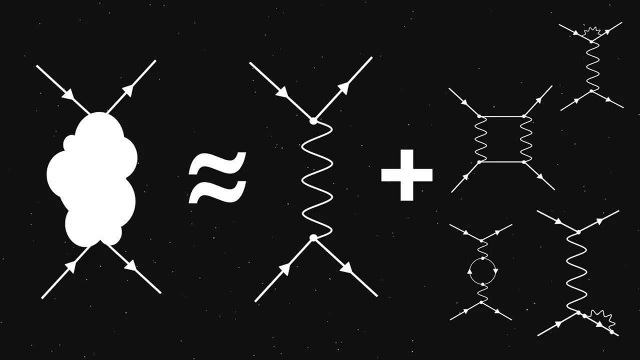 All the other and more complicated Feynman diagrams are just far less likely.